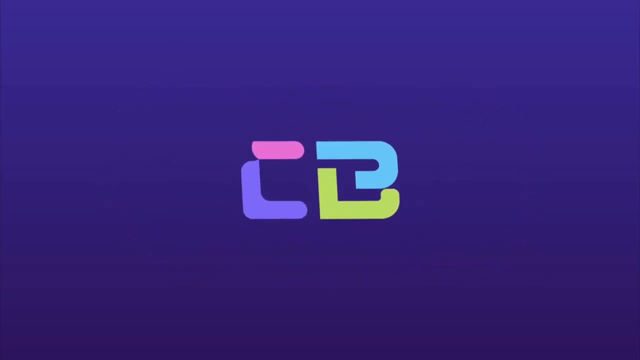 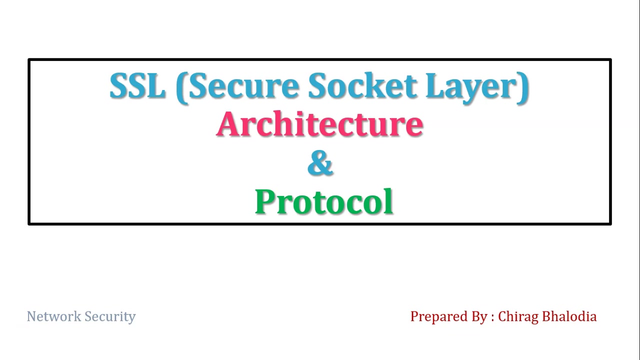 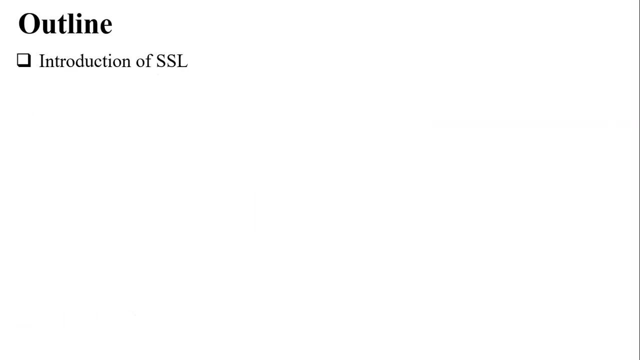 Hello friends, welcome back to my channel myself, Chirag. In this video I am going to discuss about SSL architecture and protocol Topic of network security. Let's check the outline of this video. The first topic is introduction of SSL. The second one is what? 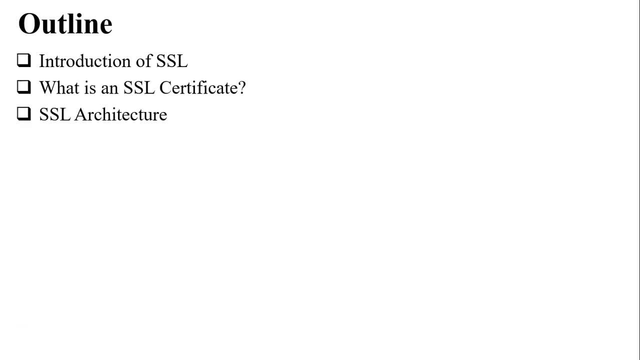 is an SSL certificate, The third one is SSL architecture And the fourth one is SSL protocols. Before start this video, subscribe me on YouTube, And all the video materials are available on my blog, chiragbalodiacom. Let's start with the first topic: introduction of SSL. 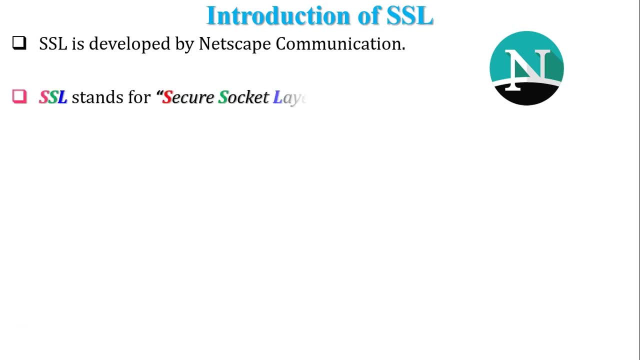 SSL is developed by Netscape Communication. SSL stands for Secure Socket Layer. So here the question is: what is SSL? SSL is a protocol for establishing secure links between network computers, So it means SSL creates secure links between network computers. So it means SSL creates secure links between network computers. So it means SSL creates secure links between. 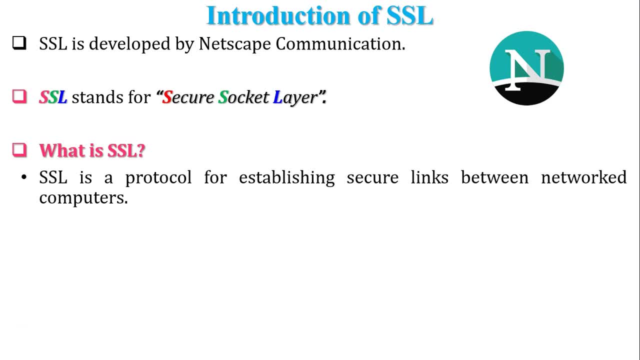 a secure network between client and server during the communication. Next purpose of SSL: SSL achieves all the security goals in internet communication. Security goals means data confidentiality, data authentication and data integrity. SL is the predecessor to the TLS. Nowadays, TLS is used instead of the SSL. You also can check the TLS encryption. 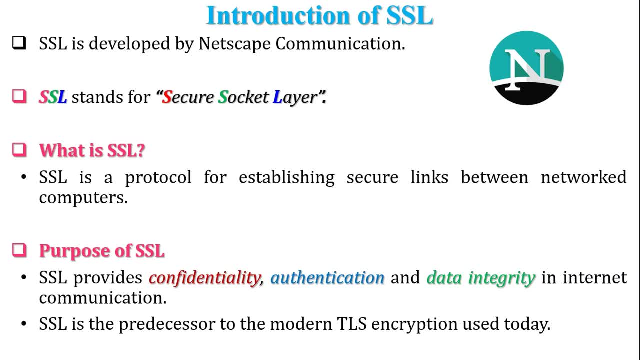 in Gmail, yahoo mail and many more websites. SSL has been used as a valuable supporting option for motors and hair件 físques, and this is the buffer that can be used to verify all the secure website use SSL or TLS encryption. Let's discuss how SSL provide the security during. 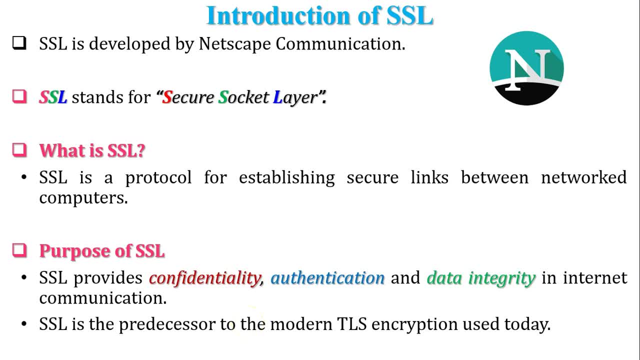 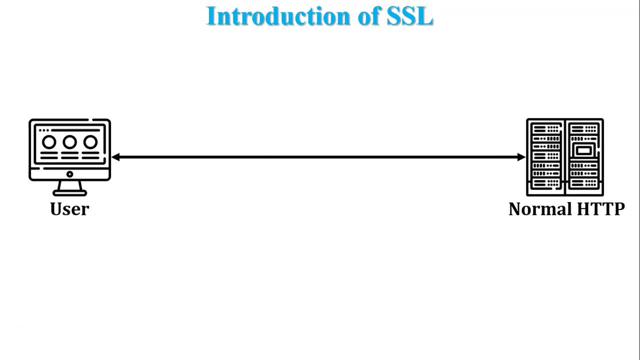 communication. Let's take one scenario to understand the concept of SSL. For example, there is one user, User want to communicate with the server, but server uses the normal HTTP. So it means the connection between the user and the server is insecure. Now we can say hacker or 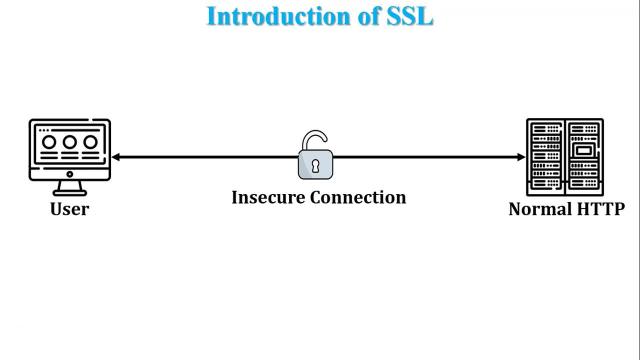 attacker can capture the message from that insecure connection. So it means hacker or attacker can impersonate as a real user to the server. So here the question is that how can we make insecure connection as a secure connection? Let's understand with one example, For example. 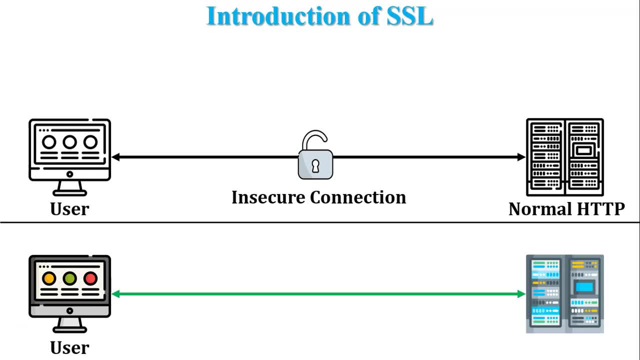 there is one user. User want to communicate with the server. In this example, server uses the secure HTTPS instead of normal HTTP. So here another question: what is HTTPS? Normal HTTP protocol is used with the SSL certificate. It is known as the secure HTTPS. So in this, 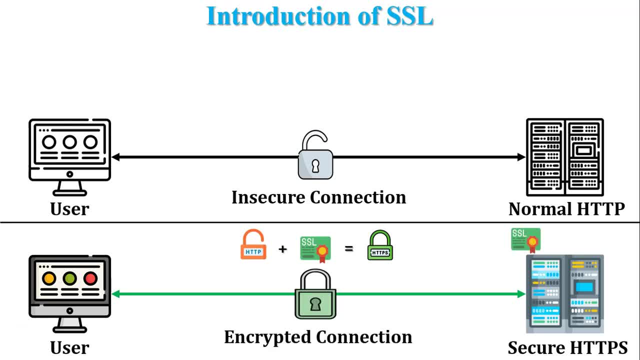 example, the server uses the secure HTTPS instead of normal HTTPS. So here another question: client and server use the encrypted connection. So, as per the definition of SSL, SSL provides the security between the network computers. So it means SSL creates secure tunnel between the user. 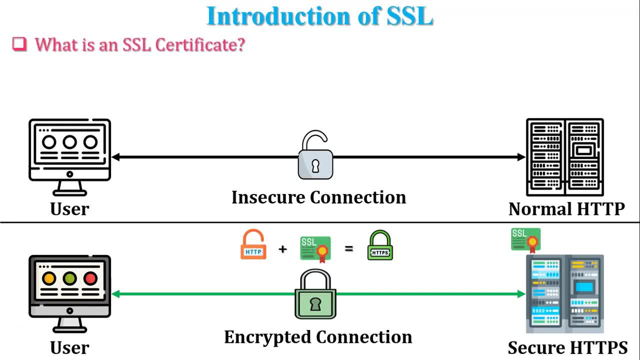 and the server. So here, another question is that: what is an SSL certificate? An SSL certificate is a bit of code which is placed on the web server that provides the security during the communication. So now, seeing this example, SSL certificate is placed on the secure web servers. So this is all. 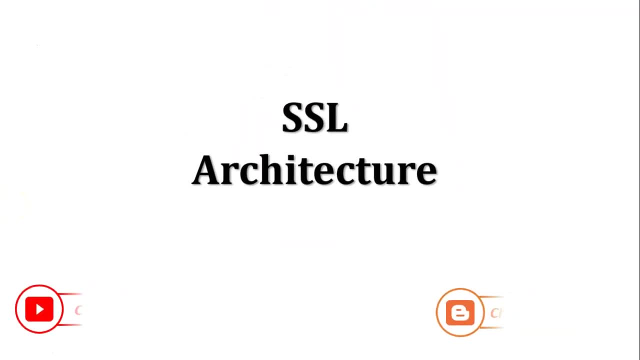 about the security between the network computers. So let's take one scenario to understand the about the security between the network computers. So let's take one scenario to understand the introduction of SSL. Next topic is SSL architecture. Let's take one example to understand the SSL. 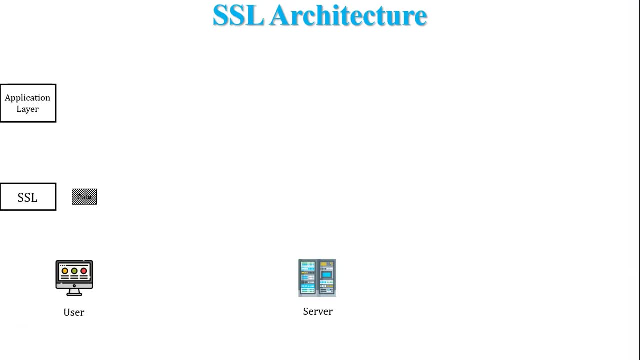 architecture. SSL encrypts the data received from application layer of the client machine and then add SSL header into the encrypted data, Then after send this encrypted data to the server side. So it means SSL is work between the application layer and the transport layer, So that SSL is also called as: 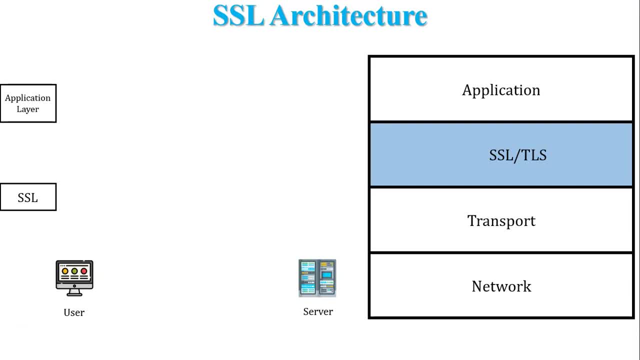 TLS. TLS stands for transport layer, So it means SSL is work between the application layer and the transport layer. security SSL is not a single protocol to perform security task. There are two layer of sub protocols which supports SSL. First sub layer consists of three protocols, So these are: 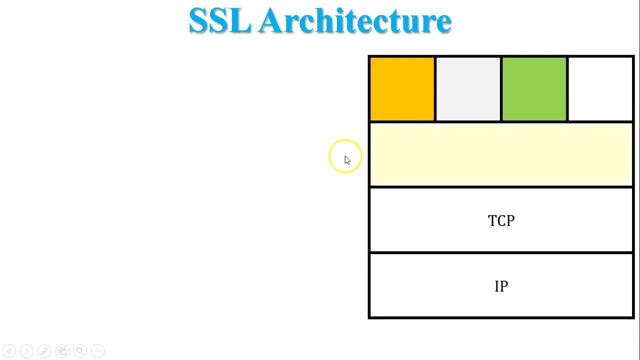 called the higher layer protocols in the SSL And there is one protocol in lower layer of SSL. The first protocol of the higher layer is SSL handset protocol. It is responsible for the connection establishment between the client and server. The next higher level protocol is SSL chain cipher spec protocol. This protocol is used of required cipher techniques for the data. 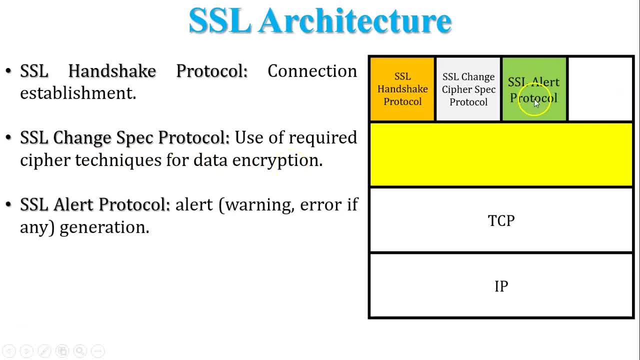 encryption. The third protocol of the higher level is SSL alert protocol. It is responsible to generate alert message. Alert message is generated when warning or error occurs before the communication is start. The lower layer protocol is SSL record protocol. It is responsible to encrypted data. 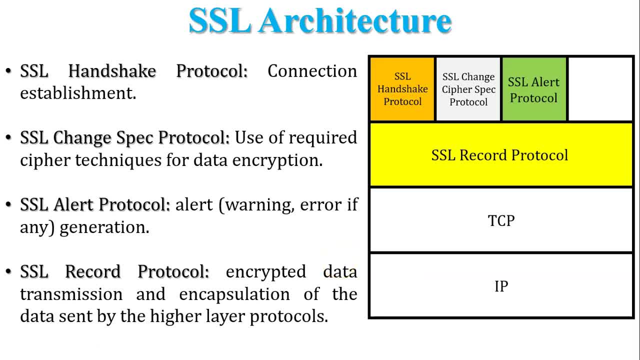 transmission and encapsulation of the data sent by the higher layer protocols. SSL record protocol is the important protocol in SSL architecture Because all kind of security is provided by the SSL record protocol during the transmission. In this architecture, the remaining field is indicate as the HTTP protocol. If you want to learn about HTTP in detail, then click on the. 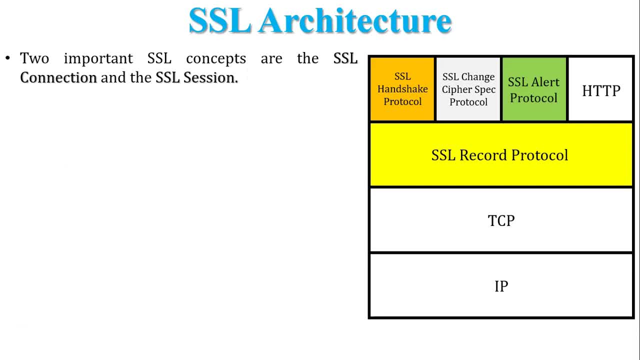 above. i button Next. there are two important terms in the SSL concept. The first one is SSL connection and the second one is SSL session. What is SSL connection? SSL connection is a transport that provides a suitable type of services. Each connection is associated with one SSL session, So 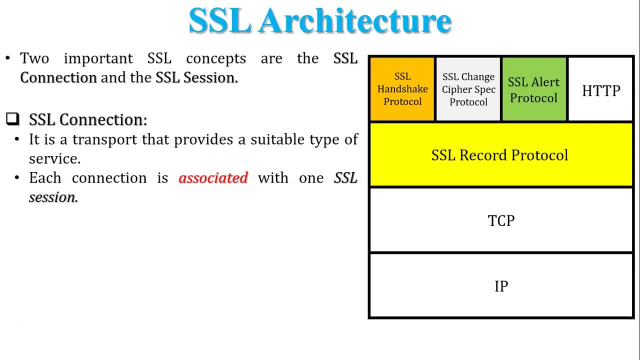 it means whenever you establish a connection, it means there is one SSL session is generated. Next, what is SSL session? SSL session is a cryptographic security parameters which can be said among multiple SSL connections Once client and server both are agree with the cryptographic security parameters. So it means security parameters are never changed throughout the connections. 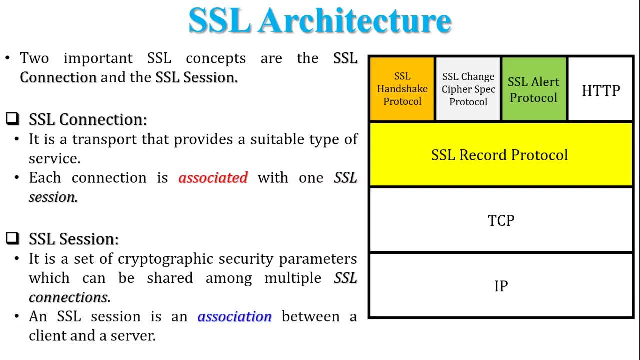 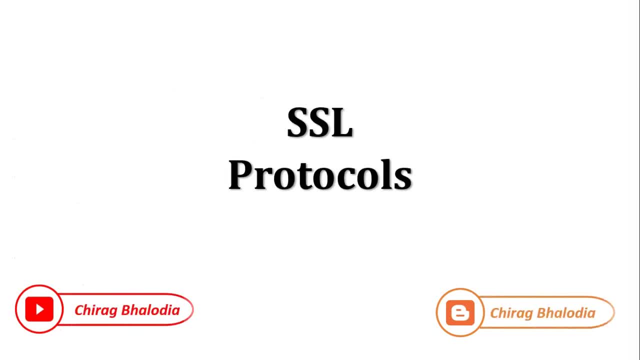 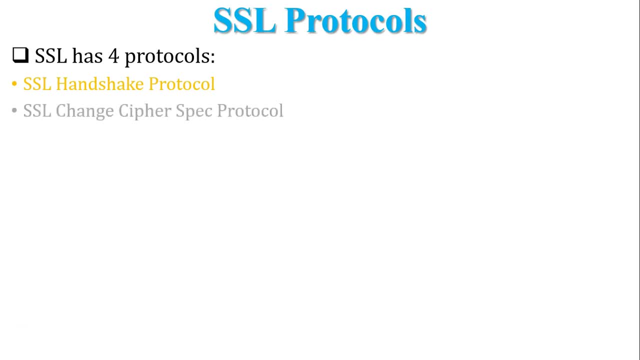 Next, an SSL session is an association between a client and a server. So this is all about SSL architecture. Let's discuss next topic: SSL protocols. SSL has four protocols. The first one is SSL handset protocol. The second one is SSL change cipher spec protocol. The third one is SSL alert. 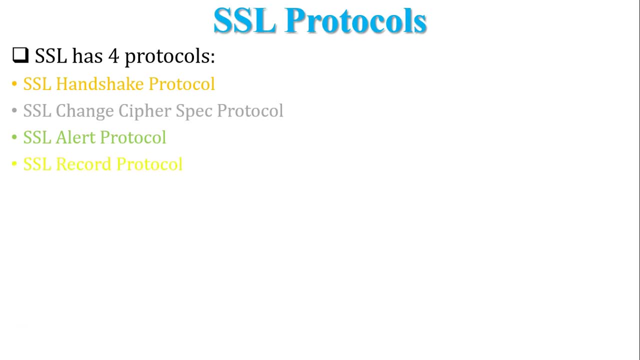 protocol and the fourth one is SSL record protocol. First three are the higher layer protocols in SSL and the last one is the SSL lower layer protocol. Let's discuss all the protocol in detail, one by one. Let's start with the first protocol: SSL handset protocol. Let's take one example to understand the SSL handset protocol. There is 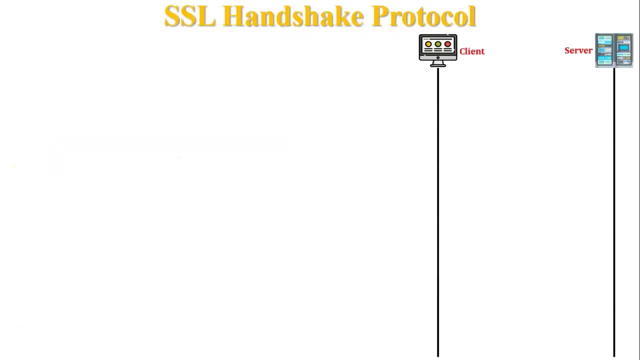 one client Client wants to communicate with the server, So client send a client hello request to the server. When server receives the client hello request, then after server send a server hello message to the client. So it is known as the phase one in SSL handset protocol. Phase one represents 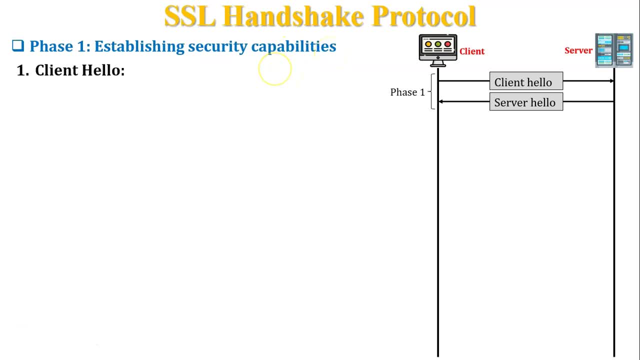 SSL sharing with client. so to save: normalmente it represents an annual easy process. So using SSL DSLeping test on the server yourself gives you an estimate for other services. The next protocol is SSL send cache. yes, This sometimes the결교, But today I am going to. 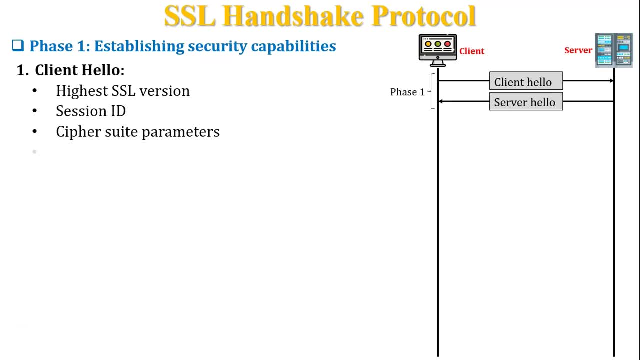 explain SSL lineUp version, which is more traditional and important to outline our service Now. first of all, this previous information is about a client message. The first parameter of the client hello message is highest SSL version. It indicates which SSL version client can support. The next parameter is sessionID. It defines the sessions. The third parameter is cipher-suit parameters. This parameter contains the list of all cryptographic algorithms which supports client system. and the last parameter is list of compression method. It indicates a list of compression methods through X at list method. Congratulations to the client. 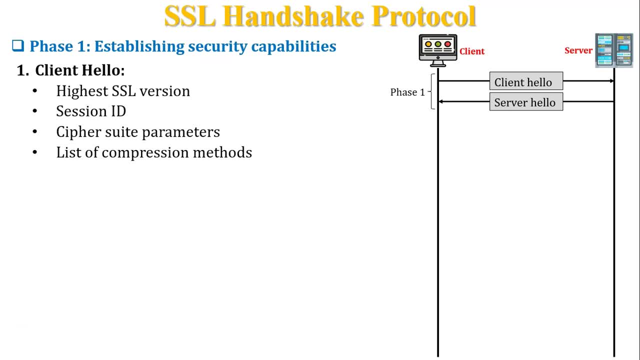 can be supported by the client. So these parameters are shared by the client with server in client hello request. Now discuss server hello message parameters. The first parameter is highest SSL version. It indicates the highest SSL version number which the server can supports. The next one is session ID. It 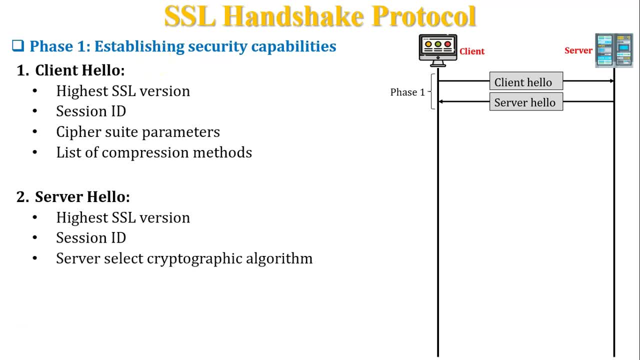 defines the session. The third one is server select cryptographic algorithm. It contains the list of all cryptographic algorithm that is sent by the client, which the server will select one algorithm from that list. The fourth one is server select the compression method: A list of compression methods sent by. 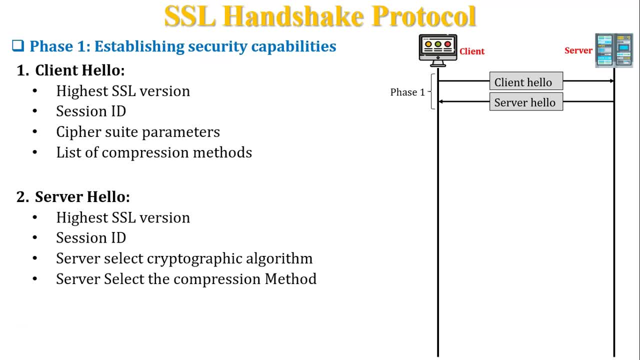 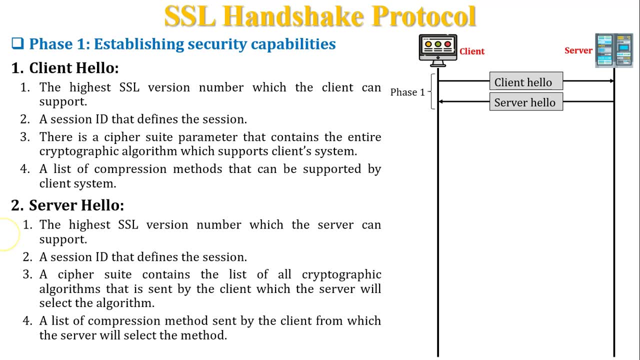 the client, from which the server will select the method from the list. So what I have discussed in phase 1 is written in this slide. You can also read from this slide: After completion of phase 1, server sends a message to the client In. 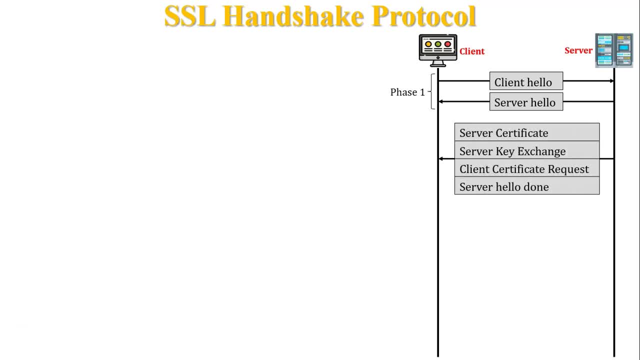 this message. There are four fields. The first one is server certificate, the second one is server key exchange, the third one is client certificate request and the fourth one is server hello done. So this message is called as phase two. Phase two represents the server authentication and key exchange. Let's discuss all the fields of phase two message. 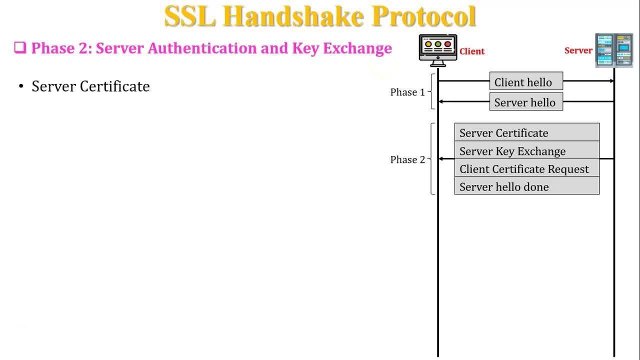 The first one is server certificate. The server sends a certificate to authenticate itself to the client. If the key exchange algorithm is Diffie-Hellman, then no need of authentication. Next field is server key exchange. This field is optional. It is used only if the server doesn't send its digital certificate. 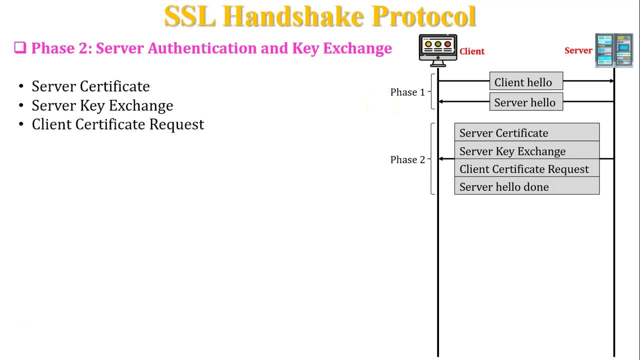 The third one is client certificate request. This field is also optional. Server can request for the digital certificate of client for authentication purpose. And the last field is server hello done. The server message- hello done is the last message in phase two. It indicates to the client that the client can now verify all the certificates received from the server. 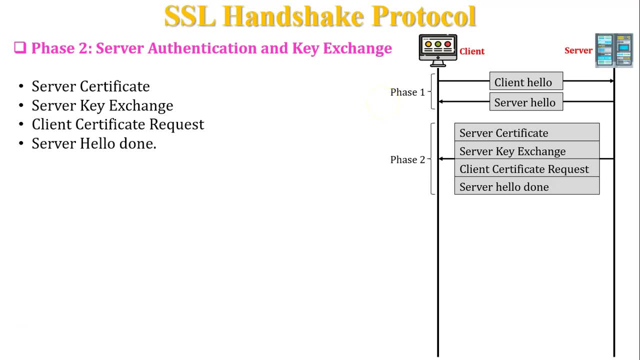 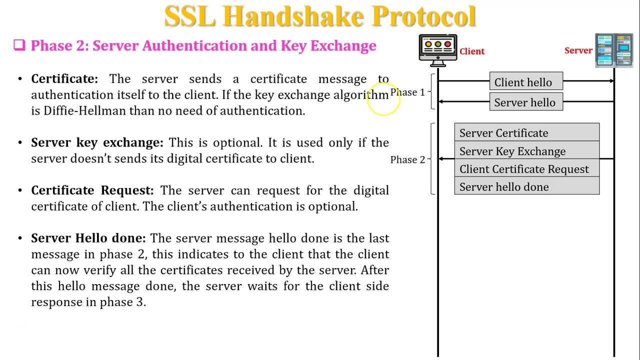 After this hello message done, the server waits for the client response. What I have discussed in phase two is written in this slide. You can also read from this slide: After completion of phase two, client send a response to the server. This client message includes three fields. 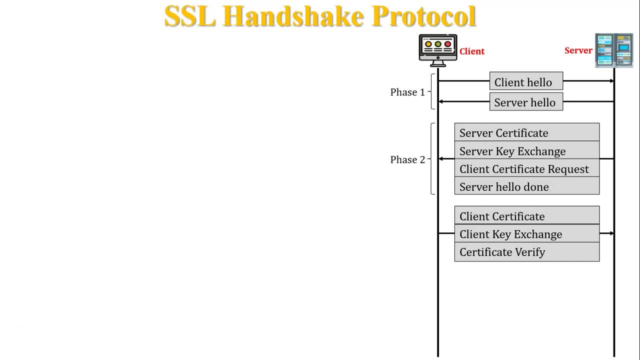 The first one is client certificate, the second one is client key exchange and the last one is certificate verify. This message, called as phase three, Share three, represents client authentication & key exchange. Let's discuss all the fields of phase three message. The first field is client certificate. This field is optional. It is only required if the server had requested for the clients digital certificate. 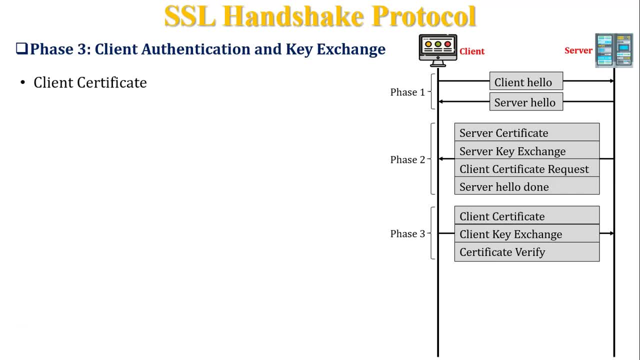 If a client doesn't have certificate, it can be send no certificate message. This can be done using之前 pigment, yellow or white box. This is an option which rationed for segment up to server's decision whether to continue with the session or to abort the session. 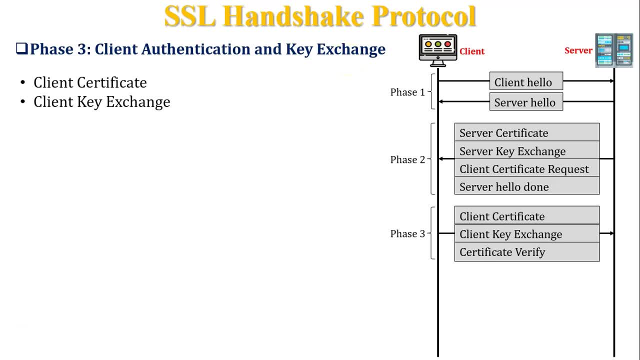 The second field is Client Key Exchange. The contents of this field are based on the key exchange algorithm between both the parties. And the last field is Certificate Verify. It is necessary only if the server had asked for the client authentication. The client has already sent its certificate to the server. If server wants, then the client has to prove. 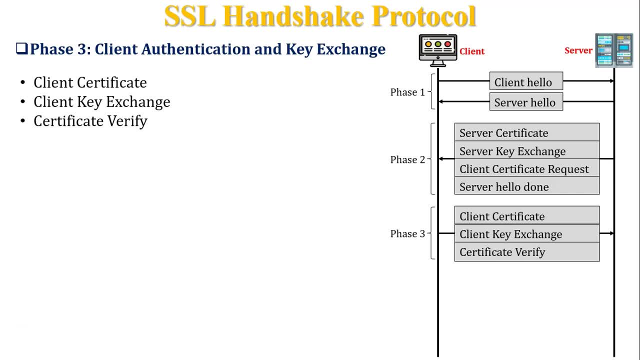 that it is authorized holder of the private key. The server can verify this message with its public key. It is already sent to ensure that the certificate belongs to the client. So what I have discussed in Phase 3 is written in this slide. You can also read from this: 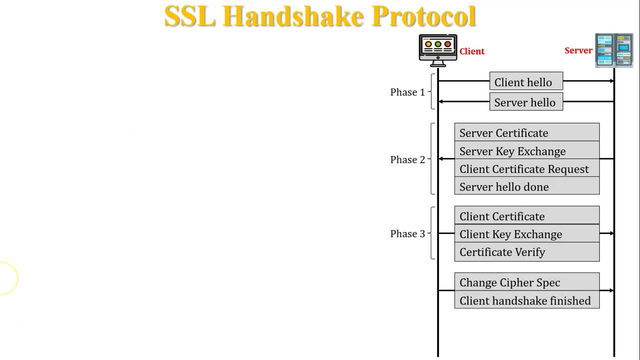 slide: After completion of Phase 3, client and server exchange the Handshake Finish message. This is called as Phase 4.. Phase 4 represents finish of handshaking. In both the messages there are 2 fields Change Cipher, Spec and. 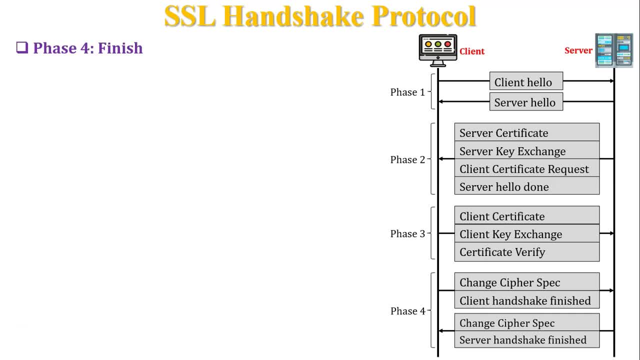 Handshake Finish. Let's discuss this field one by one. The first field is Client Side Change: Cipher Spec. It is a client side message telling about the current status of cipher protocols and parameters, which has been made active from pending state. The second field: 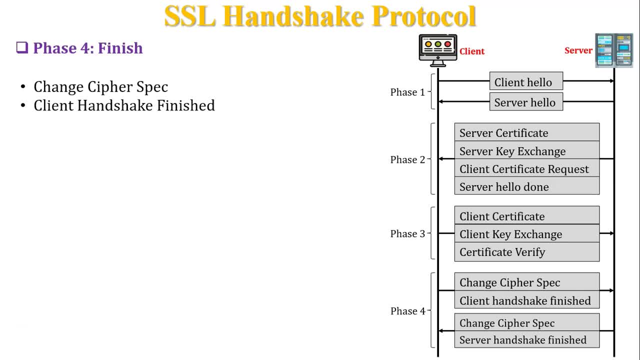 is Client Handshake: Finish This message announce the finish of the handshaking protocol from client side. The next field is Change Cipher Spec from the server side message. This message is sent by the server to show that it has made or all the pending state of the cipher protocols and parameters to active state. 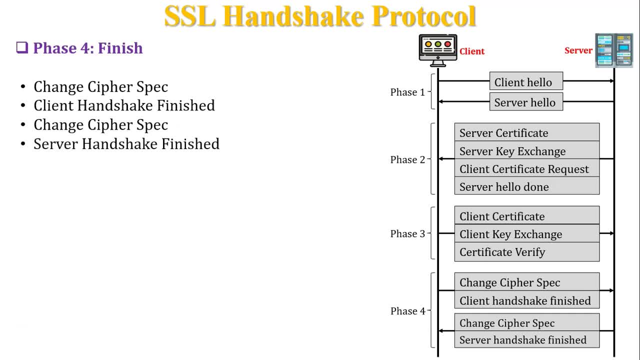 The next field is server handset finished. This message announced the finish of the handsetting protocol from server and finally, handsetting is totally completed. So it means after completion of phase 4, the connection is established between the client and server is successfully. So what I have discussed in phase 4 is written in this slide. 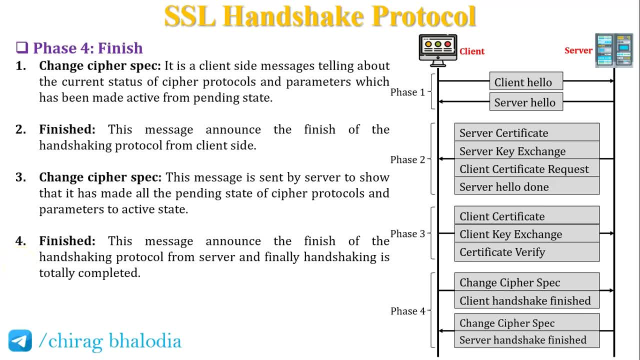 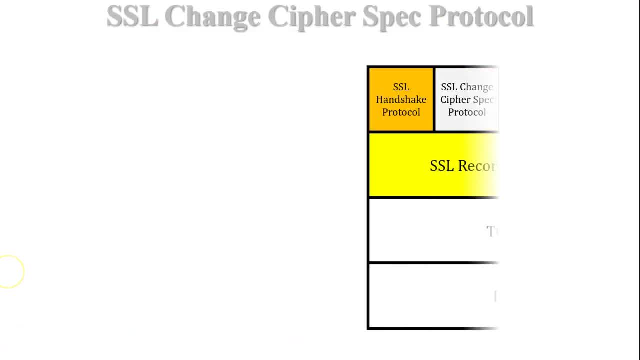 You can also read from this slide. If you have any query, you can join my telegram group, Chirag Balodia- link is given in description- and follow my blog chiragbalodiacom. Next higher level protocol is SSL change cipher spec protocol. 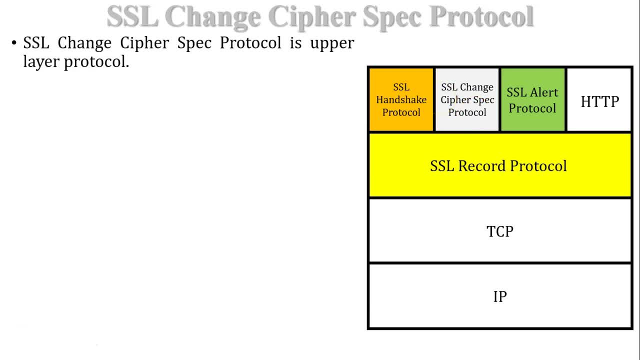 This protocol is also called as an upper layer protocol in SSL architecture. This protocol is the simplest protocol among all the protocols of SSL. This protocol consists of only single byte with value 1, as shown in this diagram. So it means SSL change cipher spec protocol occupy only 1 byte. 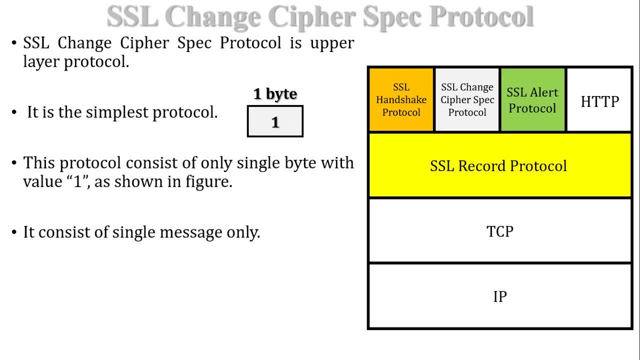 So it means this protocol is consist of a single message only at a time. The purpose of this protocol is copies pending state into the current state which updates the cipher chute to be used to this connection. So now we can say, after completion of successful handsetting between the client and server. 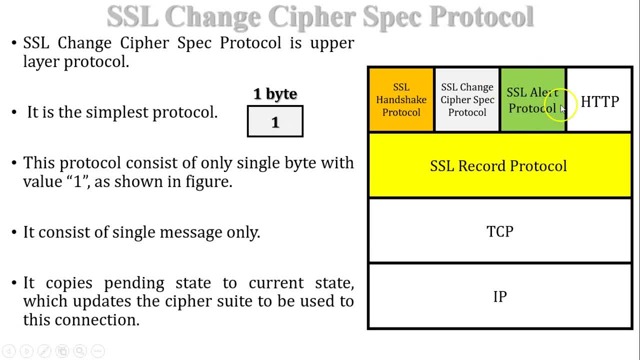 this protocol updates the cipher chute. Next higher layer protocol is SSL alert protocol. SSL uses the alert protocol for reporting error that is decided by client or server. This protocol is also called as SSL alert protocol. Next higher layer protocol is SSL alert protocol. 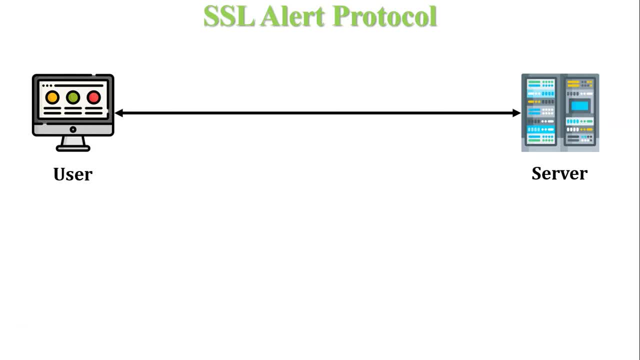 Let's take one example to understand the working of SSL alert protocol. For example: user want to send a message to the server Server. detects error or warning in that message. After detecting the error at the server side server, send alert message to the user. 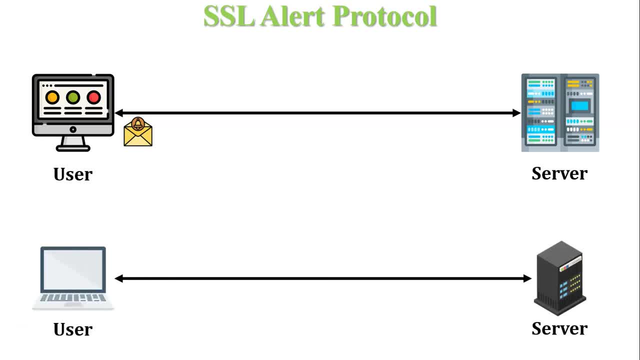 Let's take the another scenario to understand SSL alert protocol, For example. server send a message to the client and client detects the error or warning in that message. After detect error in server message, client will send alert message- alert message to the server. If error is serious, then both the 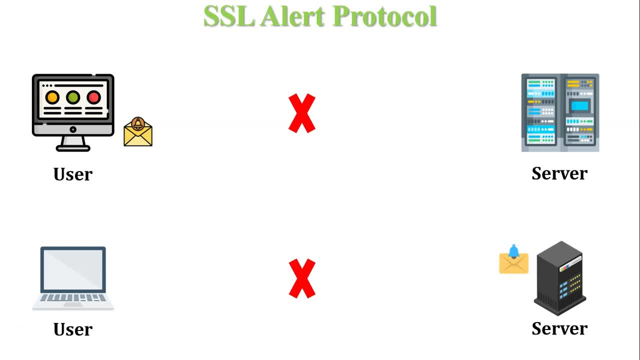 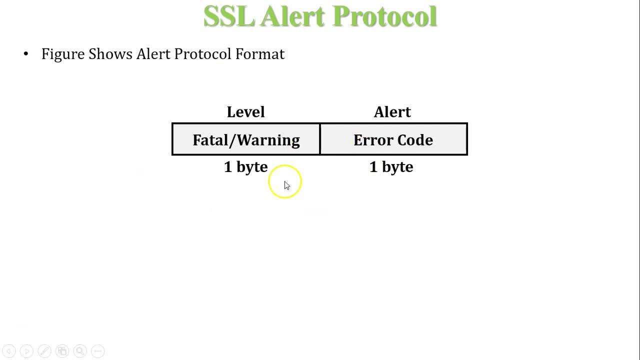 parties terminate the session. So this is all about working of SSL alert protocol. Next figure shows the alert protocol format. SSL alert protocol occupy two bytes. First one byte indicates error or warning. So it means first byte indicates either value 1 or value 2.. Value 1 indicates the warning and 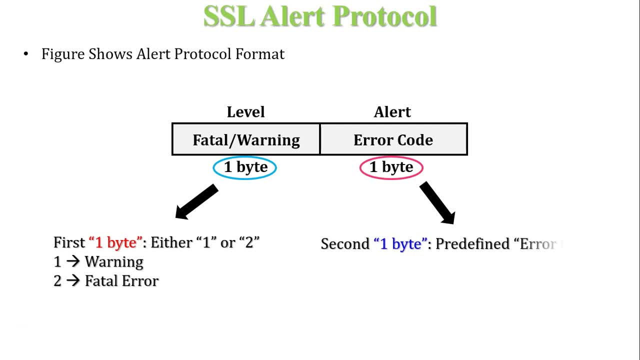 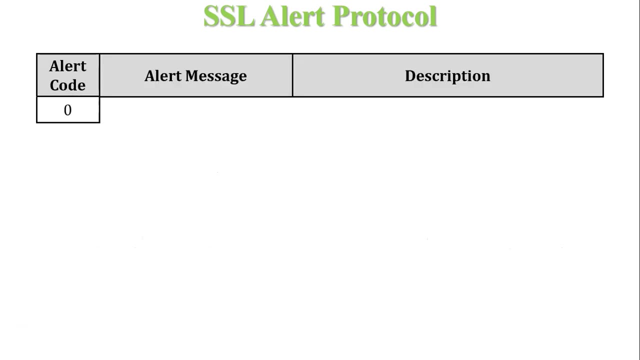 value 2 indicates the fatal error And another one byte indicates predefined error code. It means the first one byte indicates either error or warning And second one byte indicates the alert. Let's discuss different error code in SSL alert protocol. The first error code is 0.. 0 indicates close notify. 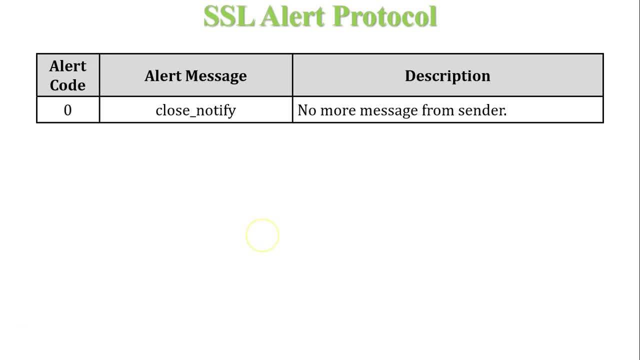 It means no more messages from the sender. So this alert message is generated by the sender only. Next alert code is 10.. It indicates the unexpected message. So it means an incorrect message is received, either server or client side. Next alert code is 20.. It indicates the bad record MAC. Here MAC means 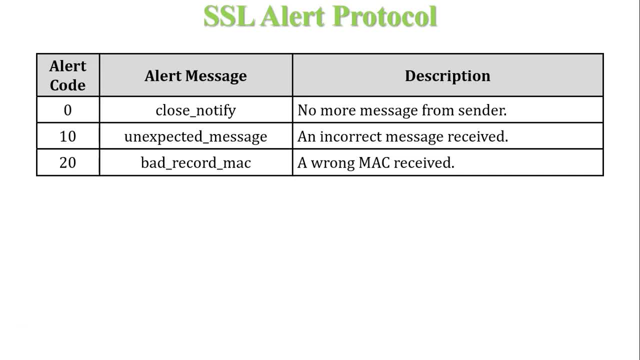 message authentication code. It indicates the wrong MAC received. Next alert code is 30.. It indicates the decompression failure, So it means unable to compress either server or client side. Next alert code is 40.. It indicates the handset failure, So it means unable to finalize handset by the sender. Next alert code. 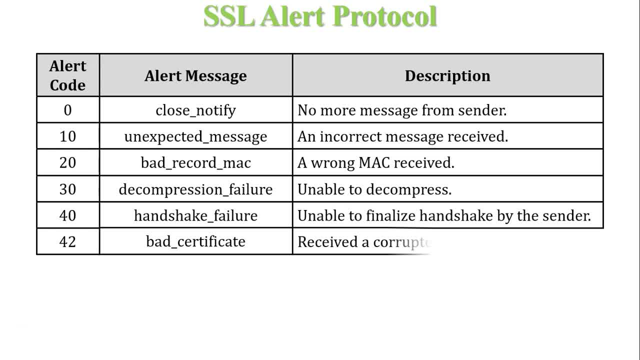 is 42.. It indicates the bad certificate. It means received a corrupted certificate, either server or the client side. Another alert code is again 42.. It indicates no certificate. It means client has no certificate to send to the server. Another alert code is again 42.. It indicates the certificate. 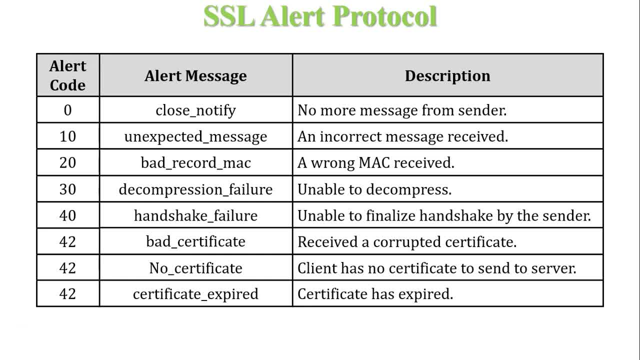 expired, It means certificate has expired, either client or the server side. So here 42 alert code is used for the 3 times. So it means whenever alert code 42 is sent, it means there is a issue in digital certificate. So this is all about SSL. 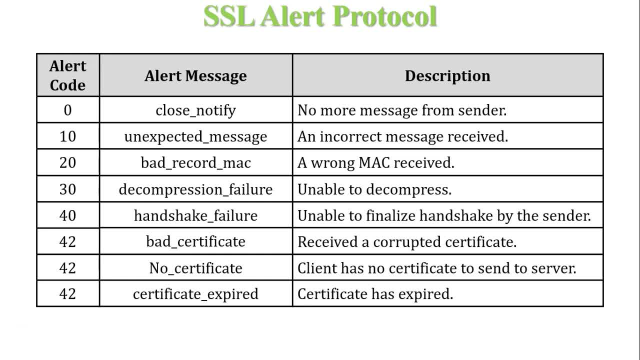 alert protocol. If you have any query regarding the SSL protocol, you can ask me in my telegram group, Chirag Balodia. Link is given in description. You can follow my blog, chiragbalodiacom. The next protocol is SSL record protocol. SSL record protocol. 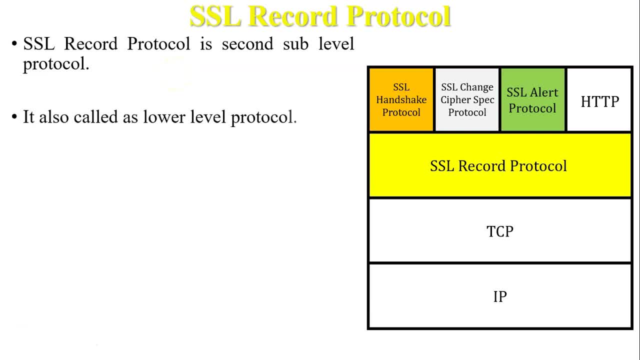 is the second sub-level protocol. It is also called as lower level protocol in SSL architecture. SSL record protocol provides following services. First one is encrypted data transmission. SSL record protocol is the responsible for encrypted data transmission during the communication between server and client. Next service: 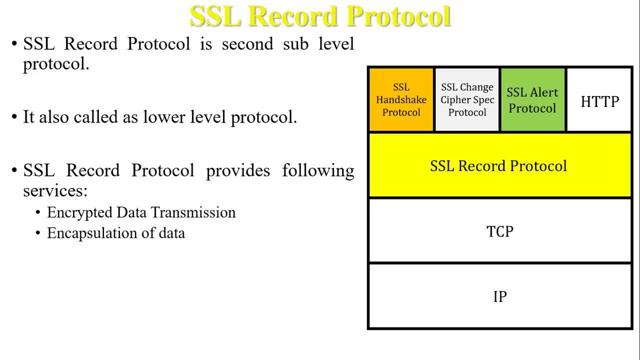 is encapsulation of data. Data encapsulation is a process by which a lower layer protocol receives data from the higher level protocol and then places the data into the data portion of its frame. Next service is data confidentiality. It can be achieved by using the secret key, which is already defined by 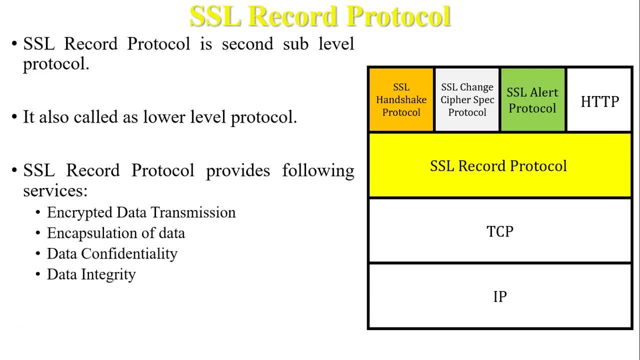 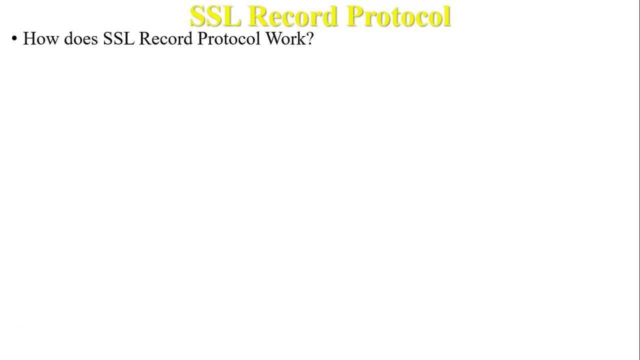 handset protocol. Another service is data integrity. Message authentication code is added with data to achieve the data integrity. So this kind of services are provided by the SSL record protocol. Next, how does SSL record protocol work? Let's take one example to understand the working of SSL record protocol. 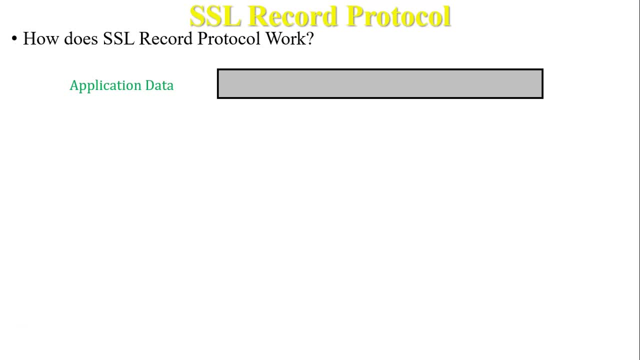 For example, this is the application data. This data is divided into the blocks before sending, So this is called as fragmentation of data. In this process, the original message is broken into the blocks before sending. The size of each block is less than or equal to. 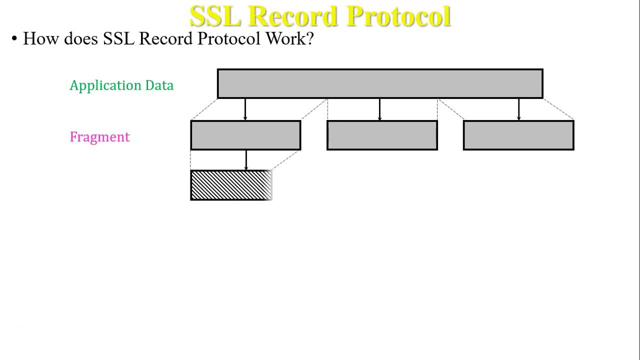 2 raised to 14 bytes. After fragmentation, the fragmented blocks are compressed, So this process is called as compression. This process is optional, but it should be noted that the compression process must not result into the loss of original data. After compression, message authentication code is added In this process a 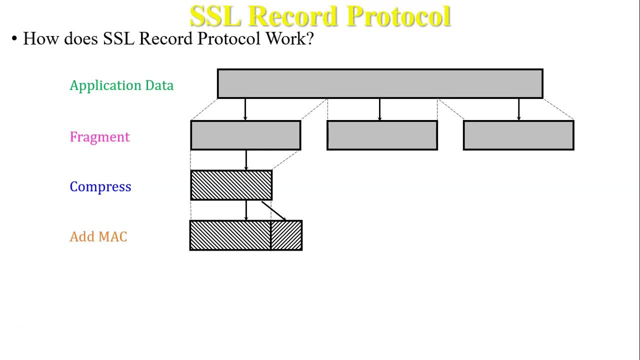 short piece of information is used to authenticate a message for integrity and assurance of the message, MAC is generated from the compressed or fragmented data block. After addition of MAC, the whole block is encrypted. In this process, the overall steps, including message, is encrypted using the symmetric key, but the encryption 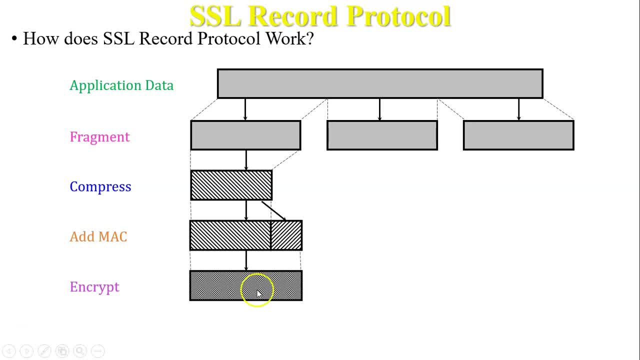 should not increase the overall steps. So it means, after encryption of data, the size of ciphertext block is same as the plaintext. After encryption of data, SSL record header is appended. So this is the working of SSL record protocol. Let's discuss SSL record. 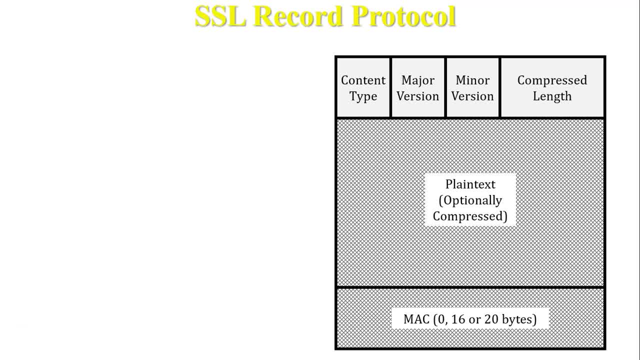 header format. This figure shows the SSL record protocol format. In this diagram, the first row indicates the SSL record header and the remaining portion is encrypted message. So following are the components of SSL record header format. The first component is content type. It indicates specify which protocol is used for. 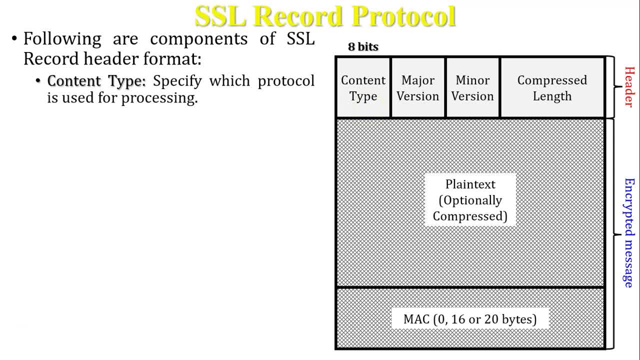 the processing Content type occupy 8 bits in SSL record header. Next, two components are major version and minor version. For example, SSL version 3.1 is used during communication. It means 3 indicates the major version and 1 indicates the minor version. Major version and minor version occupy 8 bits each.